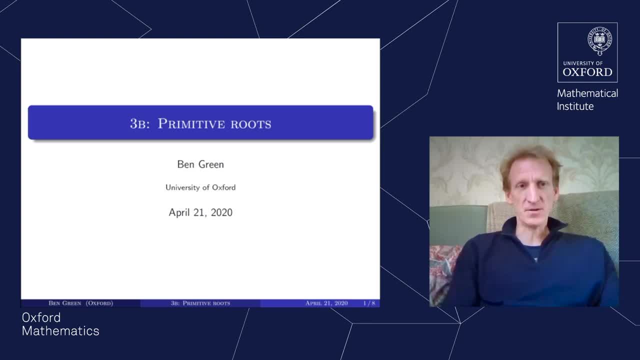 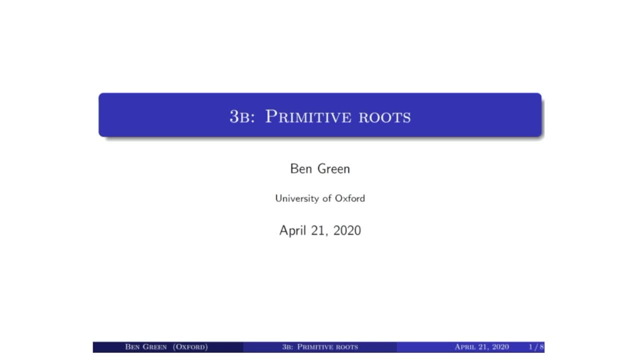 we're trying to deal with things in these very unusual times, Right, this is the second section in chapter three of the course. Chapter three of the course is about the multiplicative group, one theorem which is the existence of primitive roots, That is to say the fact that Z mod, P, Z star. 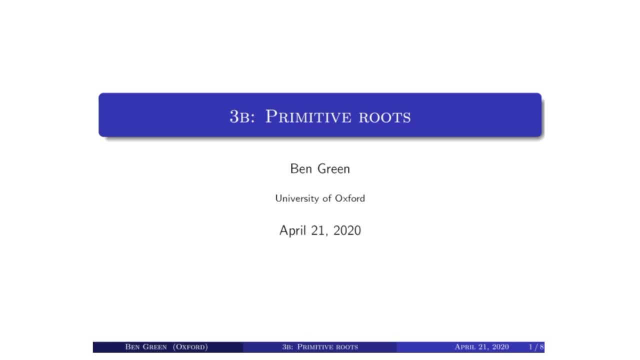 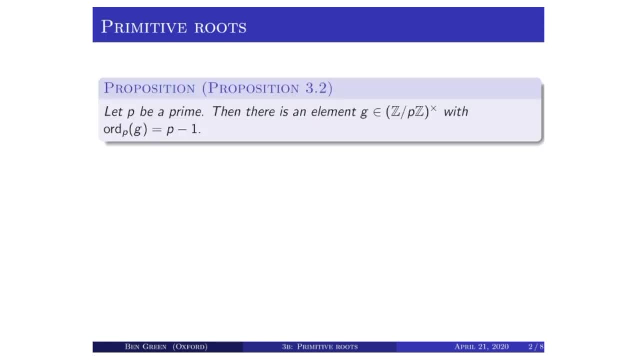 where P is a prime is a cyclic group. We'll state everything carefully later on. So this section is geared towards the proof of this, this theorem. So here is the statement: Let P be a prime. Then there is an element G. For some reason these are always called G in Z mod P, Z star. 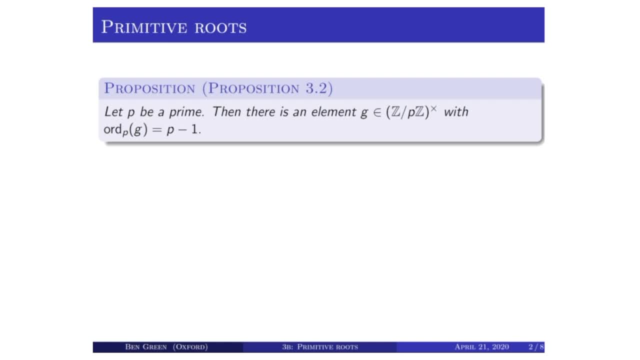 and for some reason these are always called G in Z mod, P, Z star. So that is to say the smallest positive integer n, such that G to the n is congruent to one modulo. P is P minus one. That's the largest that the order could possibly be, because by Fermat's little theorem, G to the 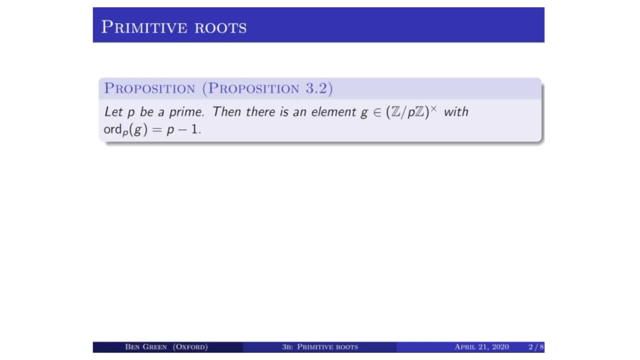 P minus one is always one mod P, no matter what G is. So it's an element G with maximal order. and equivalently, this means that Z mod P, Z star is a sine. So this is a sine of one mod P, Z star is a cyclic group, because Z mod P, Z star is a group of size P minus one, because phi of P is P. 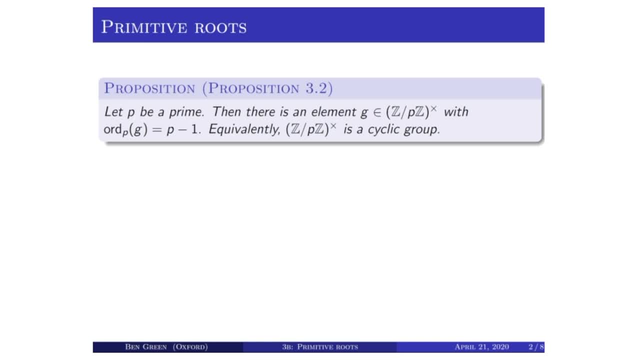 minus one, And therefore if there's an element in it of order P minus one, it must be a cyclic group of that size. So this is the main proposition that we'll be proving in this section. An element G with this property is called a primitive root modulo P, And we use that. 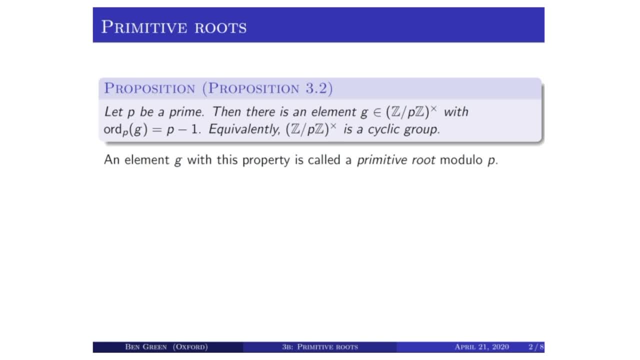 word interchangeably for either an integer G whose reduction mod P has this property, or for an element of Z mod P, Z star with this property. Now, so if G is a primitive root, then a complete list of the elements of Z mod P, Z star is: 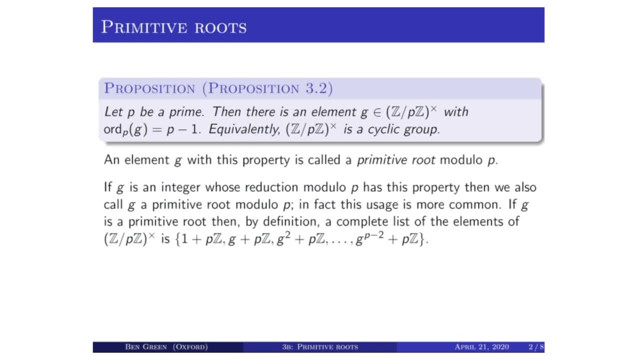 G, G squared up to G to the P minus two and one, or more accurately, the cosets of P Z by those elements. So one plus P Z, G plus P Z, G squared Plus P Z up to G to the P minus two plus P Z. 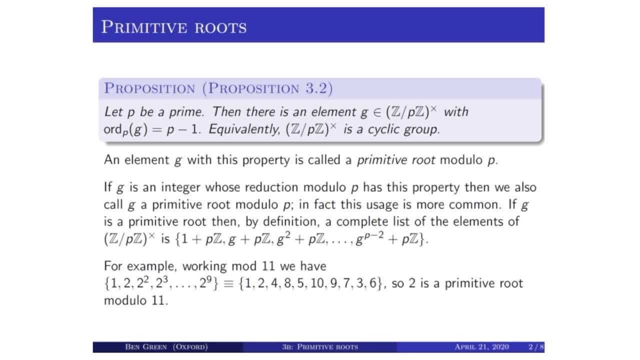 Let's have a look at a little example. So when P is 11, it turns out that two is a primitive root modulo 11.. And that's because one, two, two squared, two cubed, and so on, up to two, to the nine turn out. 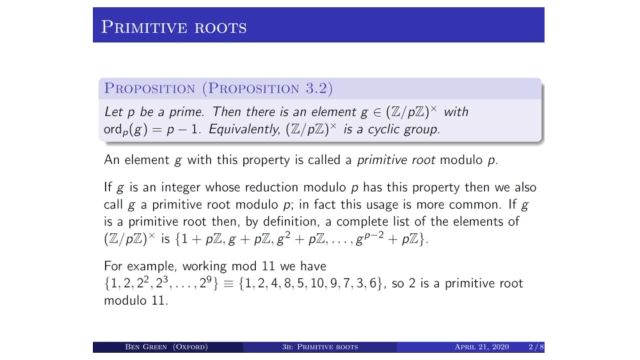 to be distinct elements, modulo 11.. And so that is a generator for Z mod 11, Z star, which is a cyclic, cyclic group of order 10.. So those are the key statements of the process of the sequencing. Now, before we get to the proof of the proposition itself, we need to take a detour into some 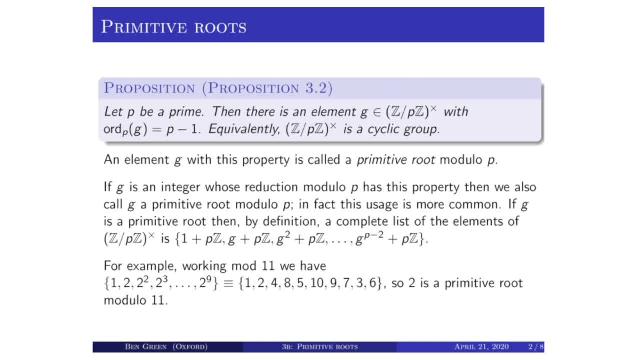 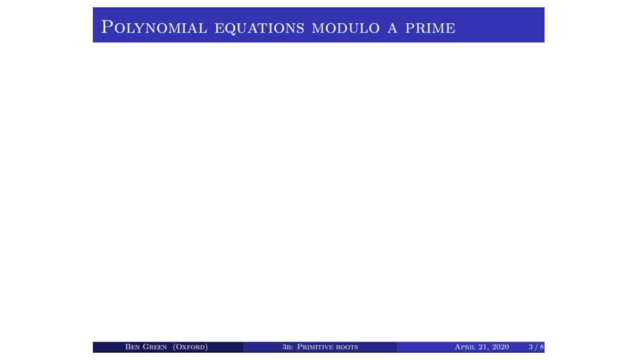 results from ring theory about roots of polynomials, some of them general and some of them more specific to the setting at hand. So let's have a look at polynomial equations modulo prime. So I think you all know the fact that quadratic equations over the reals have at most two. 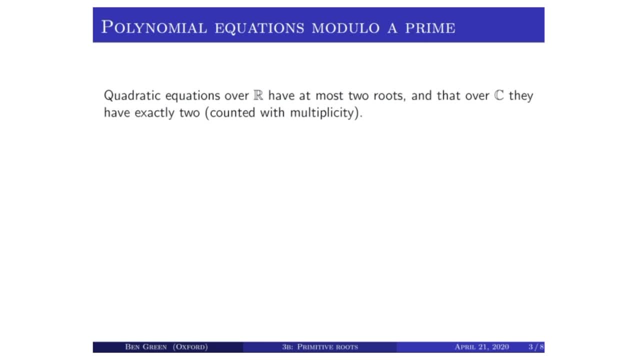 roots, Sometimes two, sometimes none, And over the complexes C they have exactly two roots. So I'm going to use one of them, and I'm going to use one of them, and I'm going to use one of them. So let's see if I can actually do it. So I've got the first one. So one of the elements of this error is that the investigator can't design the'W'' vector, so let's do the couldn't'. 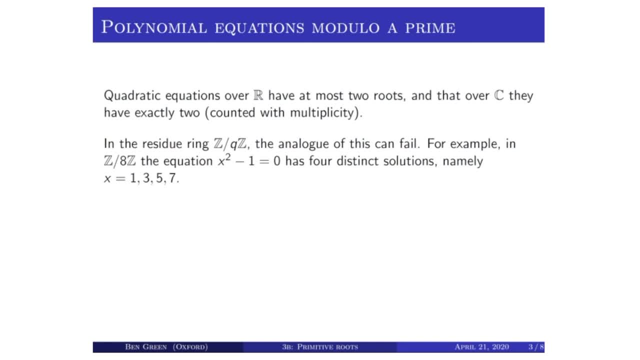 roots counting with multiplicity, But the analog of this in Z mod QZ, the ring Z mod QZ, can fail. So for instance, if Q is 8, the equation X squared equals 1, has four solutions: modulo 8,. 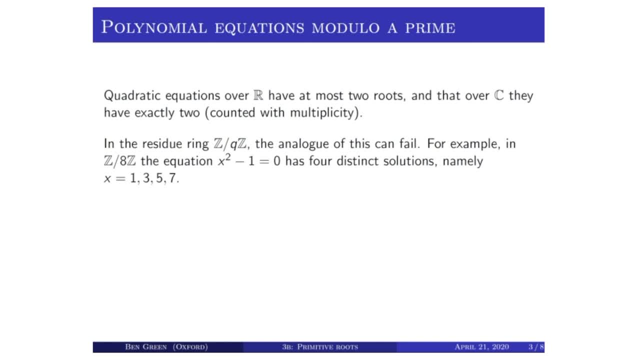 namely X equals 1,, 3,, 5 and 7.. So for all of those values of X, X squared is congruent to 1 modulo 8.. And so this fact that an equation of degree two has at most two roots. 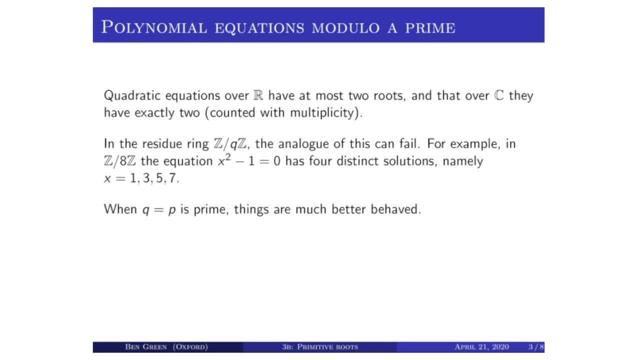 is not a fact in Z mod QZ in general, But it is true when Q is a prime. So over Z mod PZ, quadratic equations have at most two roots, And the key thing here is that Z mod PZ is actually an integral domain. 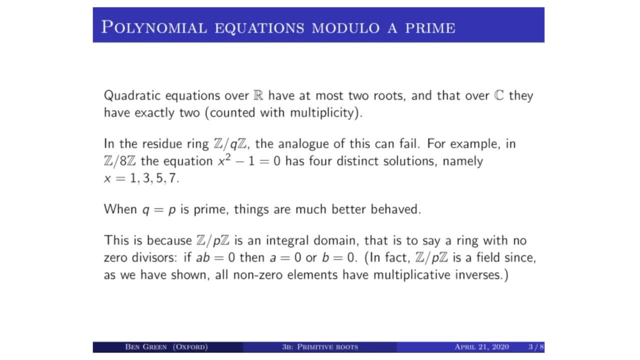 So that is to say it's a ring with no zero divisors. Or in other words, if AB equals 0, 0 in that ring. so if AB equals 0 mod P, then either A equals 0 or B equals 0.. 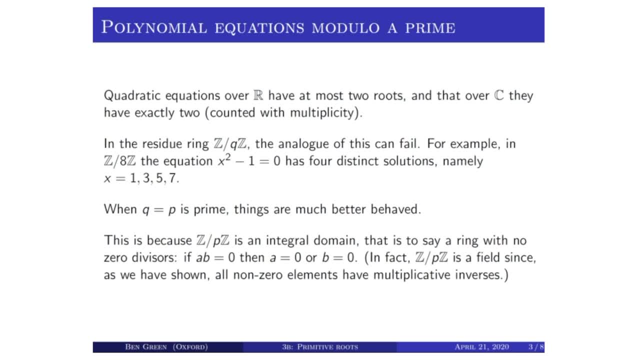 And actually, if you think about it, that is just a rephrasing of the property, P being prime. So if P divides AB, then either P divides A or P divides B And, as a matter of fact, Z mod PZ is a field. It's more than an integral domain. 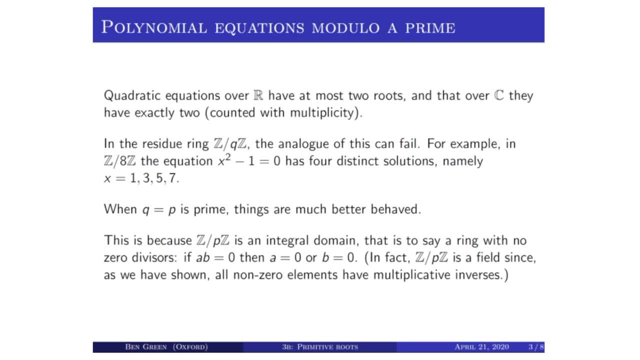 It's a field since, as we've shown, all non-zero elements have inverses. So we're working over a field, Whereas Z mod PZ is a field. So we're working over a field, Whereas Z mod PZ is a field. 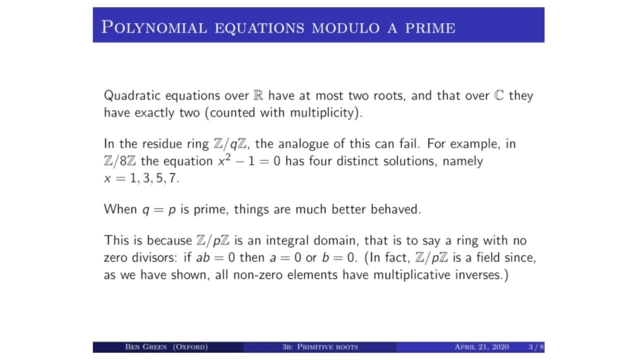 Whereas Z mod PZ is a field. So Z mod PZ is not an integral domain. It does have some zero divisors. So, for example, 2 times 4 is equal to 0 modulo 8. So it's not an integral domain and certainly is not a field. 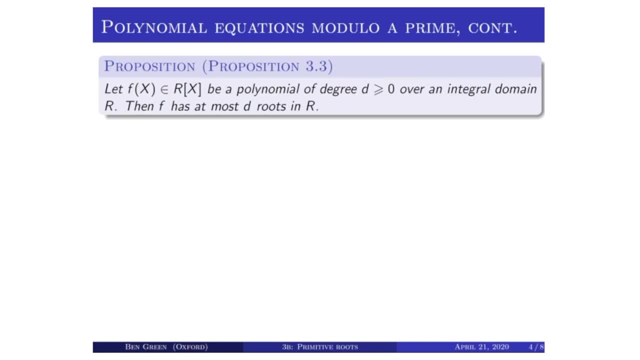 Let's state a general result about polynomial equations. So we're really interested in this result in Z mod PZ. But we'll state it and prove it in an arbitrary integral domain, R, because the proof is just the same. So let F of PZ equal 0.. 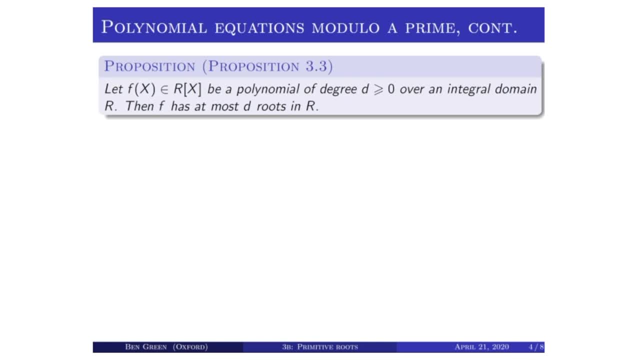 So let F of X be in the polynomial ring, big R of X of some integral domain, R, And suppose that F is a polynomial of degree d, Then the proposition is that F has at most d roots in R. So here's the proof. 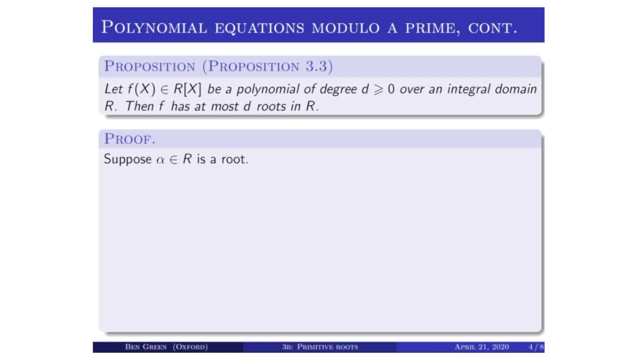 So this is at most d distinct roots. I'm not talking about multiplicity here, So suppose that alpha is a root. Suppose alpha in big R satisfies, F of alpha equals 0. Now, by the division algorithm for polynomials trying to write F as a multiple of X minus alpha, plus a remainder, 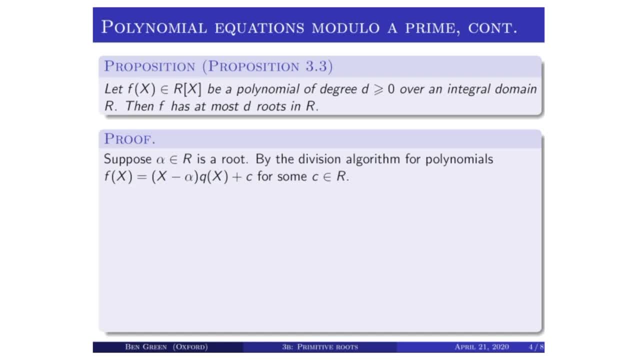 You can do that with the remainder being a constant. So you can just do this by successively knocking out terms, starting from the largest degree term of F. Take the top coefficient of Q to be such that the top coefficient of X minus alpha times Q. 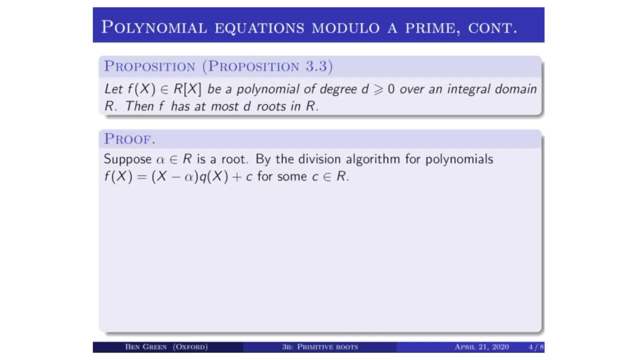 matches the top coefficient of F. That way you can just implement that quite wrong- the top coefficient of f- and then keep working down through the degrees until you have a constant left at the end. So that's the division algorithm for polynomials. No matter what alpha is not using the fact that it's a root, f of x is equal to x minus. 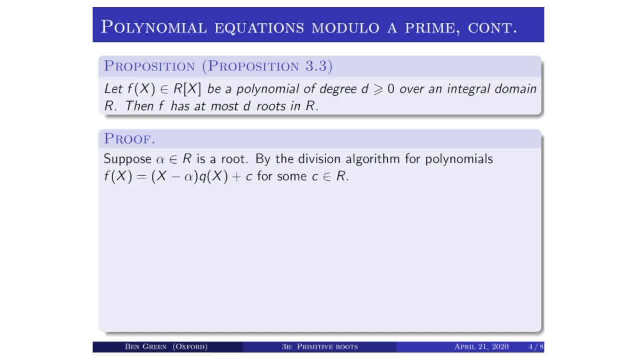 alpha times q of x plus a constant c, for some polynomial q and some constant c in this integral domain R. Now let's substitute alpha into this expression. On the left hand side we get f of alpha, which is zero by the assumption that alpha is a root of f, And on the right 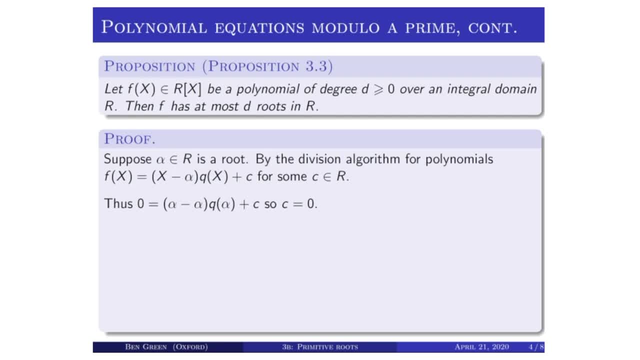 hand side, we get alpha minus alpha times q of alpha, which is zero plus c, And that must of course mean that c is zero. So we've shown the factor theorem that f of x is x minus alpha times q of x for some q. Now let's take another root of this polynomial, f. So 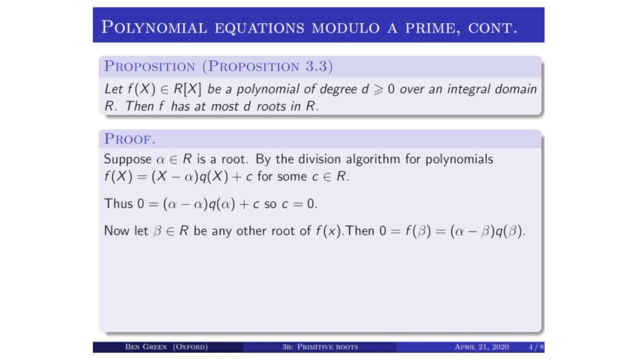 let's take another root, beta, And if I substitute it with a root of x, we get a root of x. So we get a root of x. And if I substitute it with a root of x, we get a root of x. And if I substitute it with: 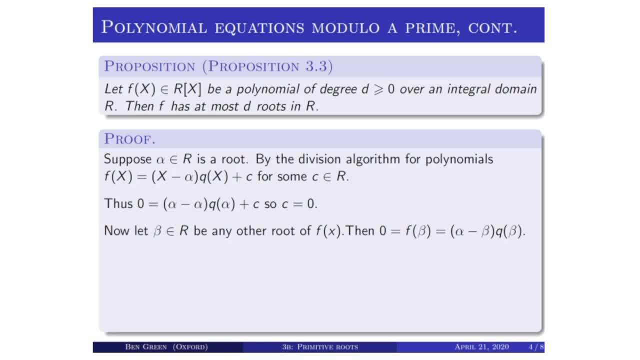 a root of x, we get a root of x, And if I substitute that into what I now know, f of beta is zero. And f of beta is also beta minus alpha times q of beta. But if beta really is another root, so if alpha and beta are distinct, then alpha minus beta is not zero. 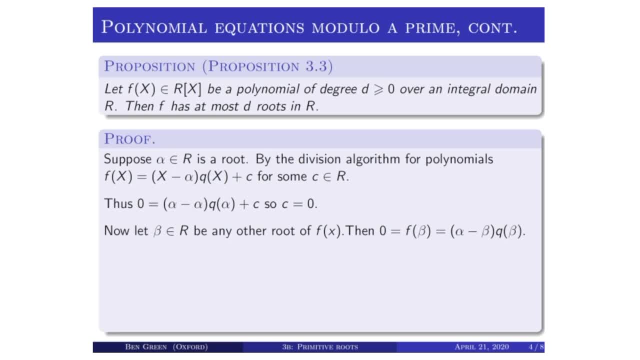 And therefore q of beta is zero, And this is the point at which I've used the fact that big R is an integral domain. So I've got the product of two things, which being equal to zero, And I'm forced to conclude that one of the two things is an integral domain. 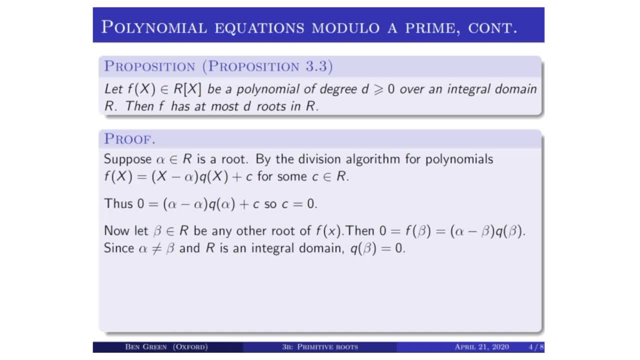 And I'm forced to conclude that one of the two things is equal to zero, And it's definitely not alpha minus beta. So q of beta is zero. And now I can proceed by induction on the degree. So q is a polynomial of degree d minus one, And so by induction has at most d minus. 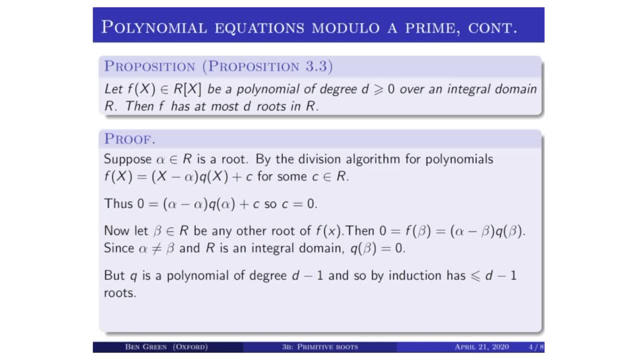 one roots, And therefore the roots of f being the roots of q, together with alpha, that has at most d distinct roots. So by induction on the degree I've proven the proposition, And therefore the roots of f being the roots of q, together with alpha that has at most 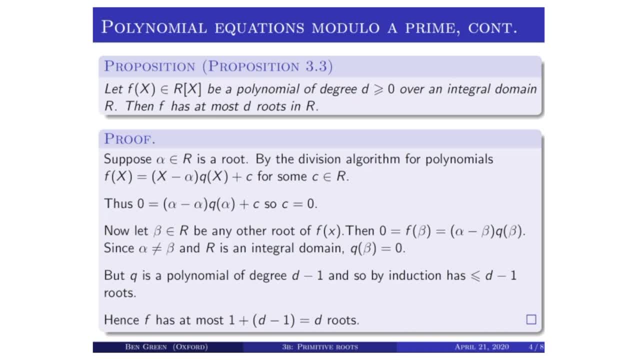 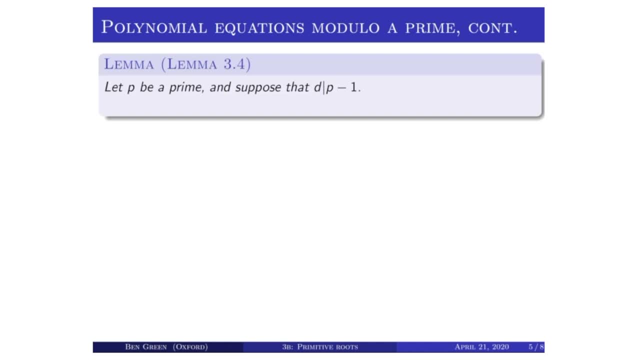 p minus one plus d minus one equals d roots. So that's polynomial equations modulo over an integral domain. Now let's be a bit more specific to z mod p, z. So let's state another lemma. This will be another lemma about polynomial equations. 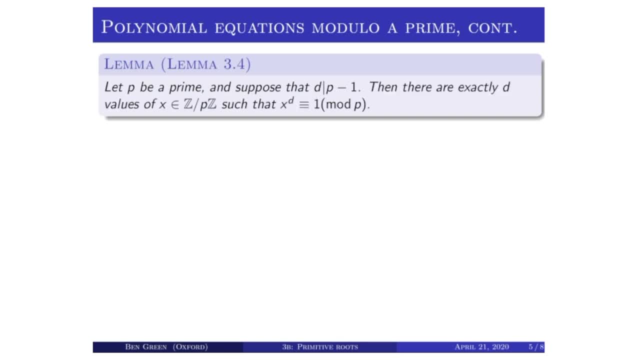 So suppose that p is a prime And suppose that d divides p minus one, And the lemma is that there are exactly d values of x in z mod p, z, such that x to the d is congruent to one modulo p, Not at most d, exactly d. 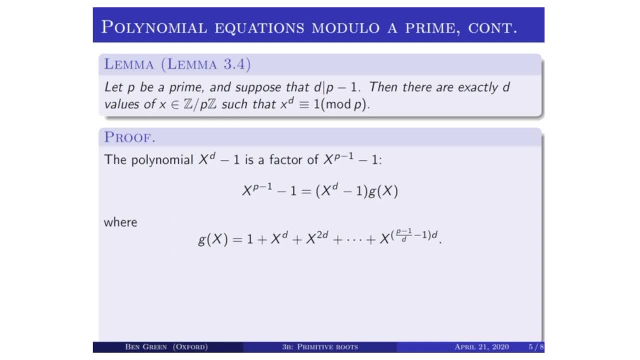 And here's the proof of that. Well, the key observation is that x to the d minus one is a factor of x to the p minus one minus one. So this is a general property of polynomials. If a divides b, x to the a minus one divides x to the b minus one, And you can write down: 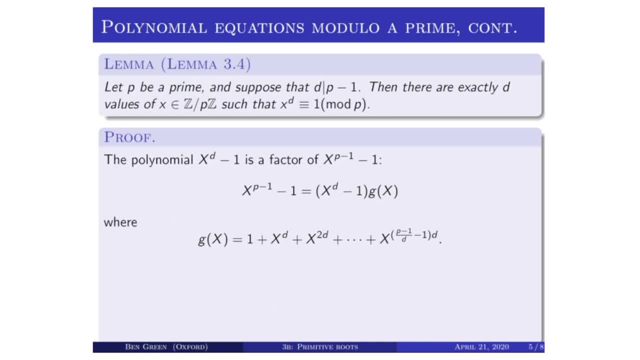 the factorization explicitly in this case. So x to the p minus one minus one is x to the d minus one times a polynomial g of x, where g of x is just one plus x to the d plus x to the two d plus up to x to the p minus one over d minus one times d. 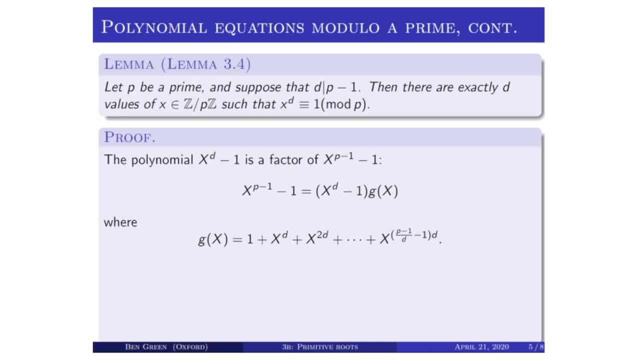 There's a very explicit factorization. Now here's the crucial observation: The polynomial on the left, x to the p, minus one minus one, has a lot of roots by Fermat's Little theorem. In fact, everything in z mod p, z star is a. 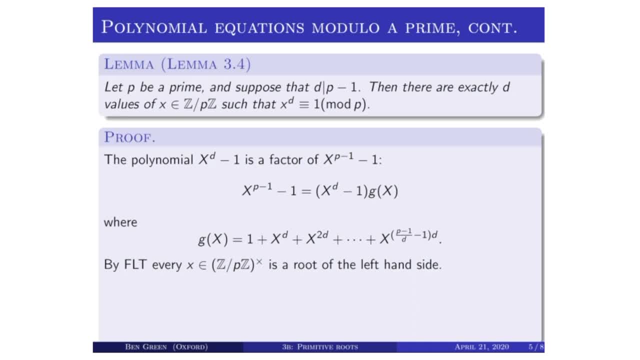 root of that, And that's p minus one, different elements. So x to the p minus one minus one, modulo p. So in z, mod p, z has p minus one distinct roots, And they must also of course, be roots of the right hand side of the displayed equations. 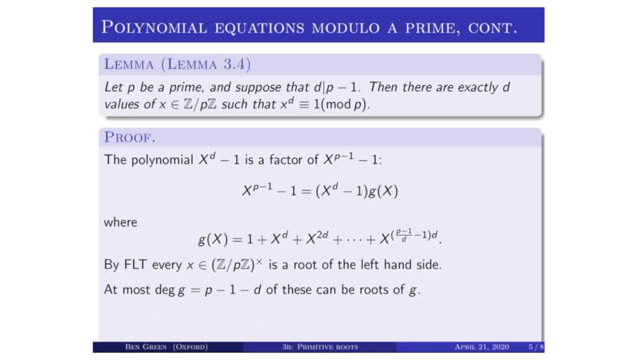 They've also got to be roots of x to the d minus one times g of x. But g is a polynomial of degree- p minus one minus d- And therefore, by the result I showed on the last slide, it can't have more than p minus one minus d roots. 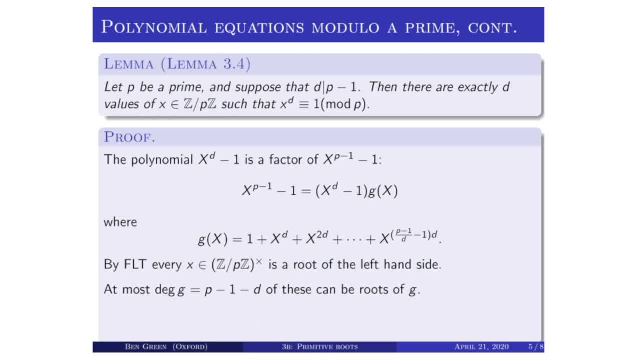 So if the p minus one roots of the left hand side x to the p minus one minus one, no more than p minus one minus d of them can be roots of g, And that means that the other d roots have got to be roots of x to the d minus one. 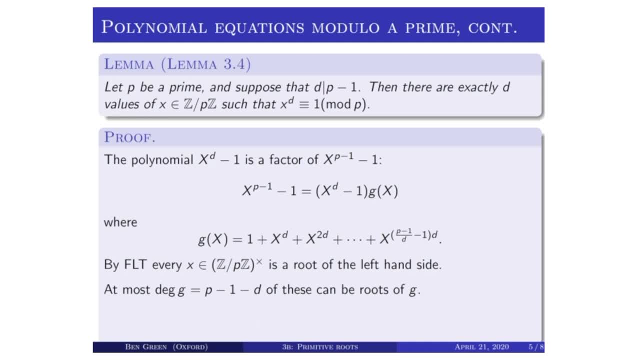 So there are indeed at least d values of x, such that x to the d is congruent to one mod, p, And in fact there are also at most d values of x With that property, again by the proposition on the last slide. 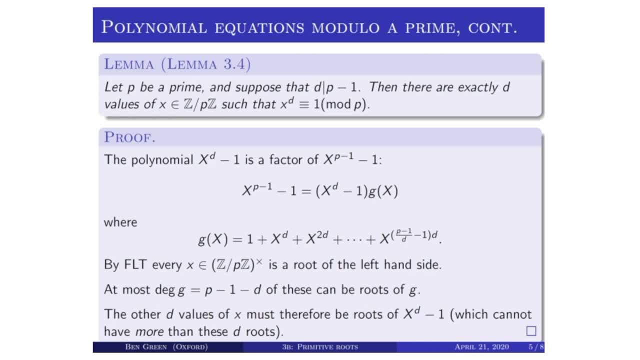 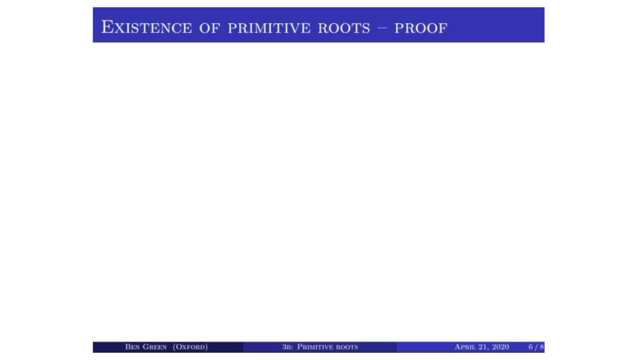 So that concludes the proof of the lemma. And this was a little bit specific, well very specific, to z modulo p, z. We've really used Fermat's little theorem here Now. then we've assembled those ingredients about polynomials. We'll turn to the actual proof of the existence of primitive roots. 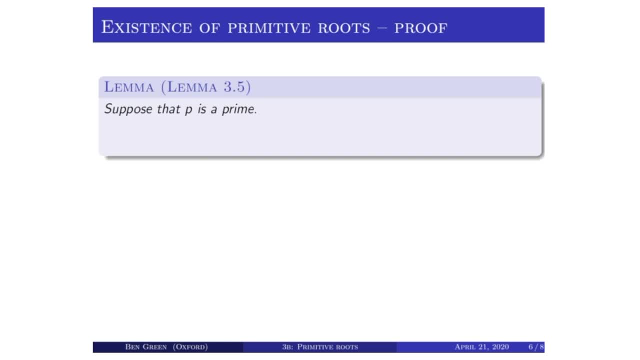 And we'll need another lemma before we really get into the heart of it. So let p be a prime, Let q be another prime, And suppose that q to the c divides p minus one for some integer c, And the conclusion is that there's an element a in the multiplicative group, z mod p, z star. 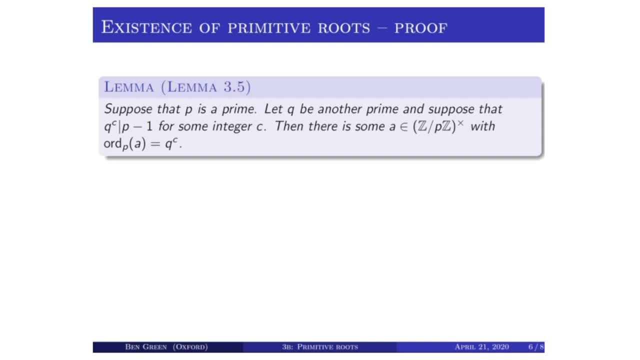 whose order is exactly q to the power c. So let's have a look at the proof of that By the lemma on the last slide, lemma 3.4.. There are q to the power c. So let's have a look at the proof of that. 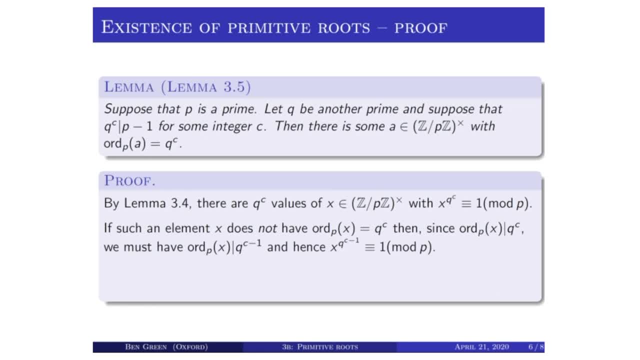 By the lemma on the last slide, lemma 3.4.. There are q to the power c, There are q to the c. values of x that do satisfy x to the q to the c is congruent to one modulo p And we just need to show that they're not all elements of strictly smaller order than q to the c. 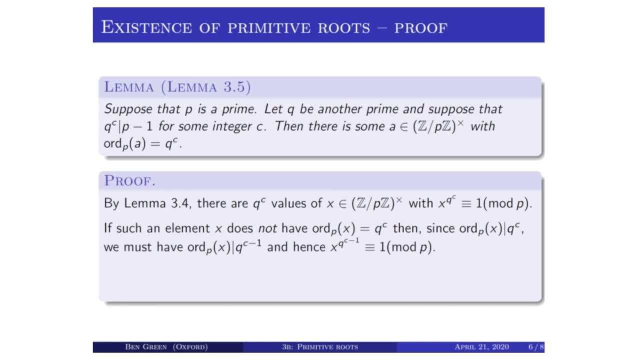 So if I've got one of those x's and if it does not have order q to the c, Then we know by the basic properties of order that its order must divide q to the c. And because q is a prime, If you've got something that divides q to the c, 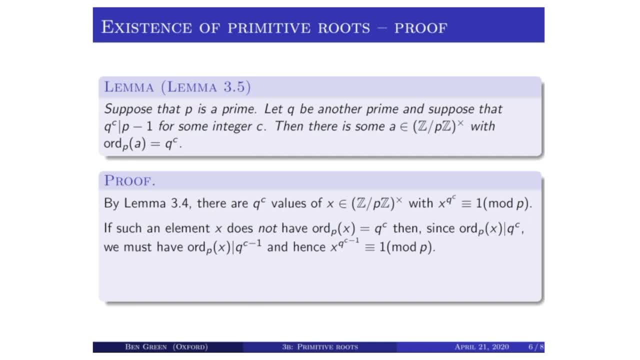 And is not q to the c, Then it must divide q to the c minus one. So if x is an element satisfying x to the q to the c is congruent to one mod p, But which does not have order q to the c. 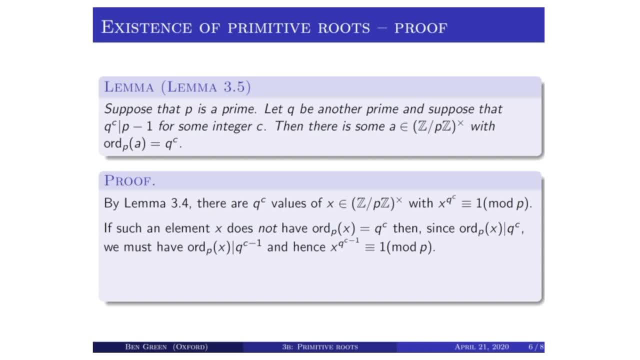 Then its order must divide q to the c minus one, And therefore that element x satisfies the polynomial equation. x to the q to the c minus one is congruent to one mod p, But that polynomial equation has at most In fact exactly q to the c minus one roots. 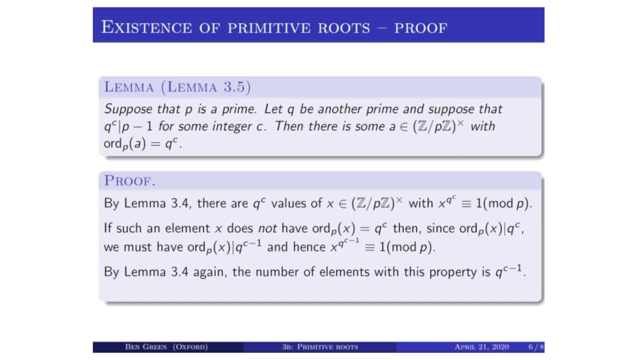 So the number of elements that have that property is q to the c minus one, And what this means is that of the q to the c, elements of x satisfying x to the q to the c being congruent to one mod p, Only q to the c minus one of them, which is a strictly smaller number. do not have order q to the c. 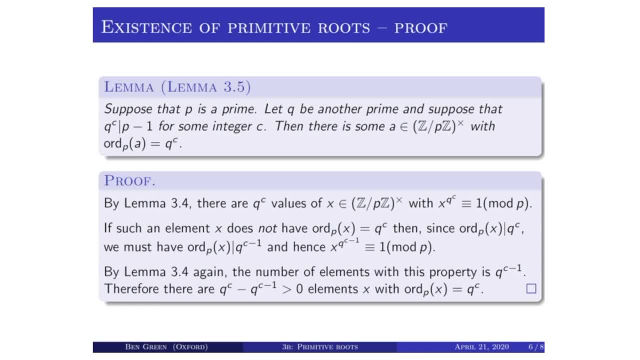 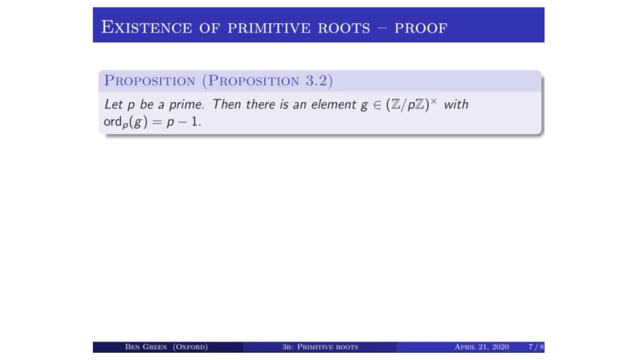 So in fact, there are q to the c minus q to the c minus one, which is a positive number. There are also elements x, whose order is exactly q to the c, and that completes the proof of the lemma. So let's continue with the proof of the existence of primitive roots. 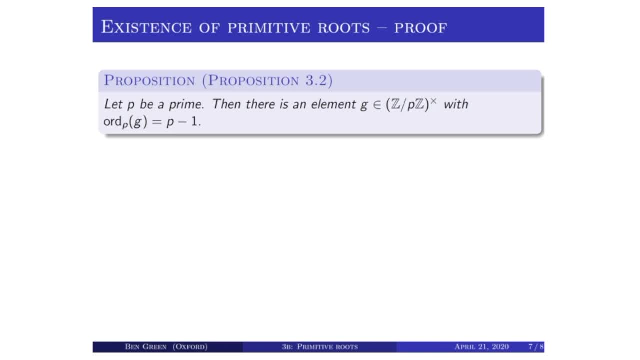 And here's just a restatement to remind you of what we're trying to prove. So this is proposition three, point two. The statement is that there's an element g in z mod p, z star, if p is a prime whose order is exactly p minus one. 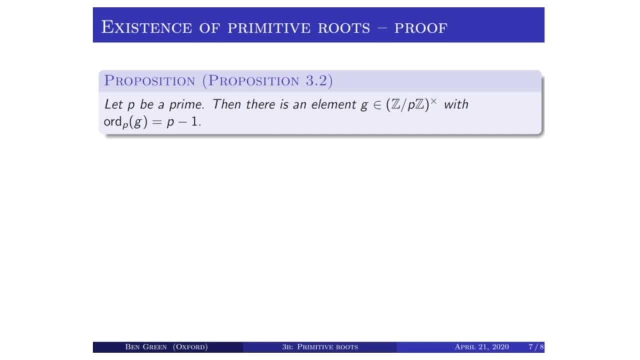 And we're just going to combine a whole load of results We've already proven. So we'll factor p minus one. Let's factor it into products of distinct prime powers, So it's q1 to the c1 times up to qk to the ck, where the qi are distinct primes. 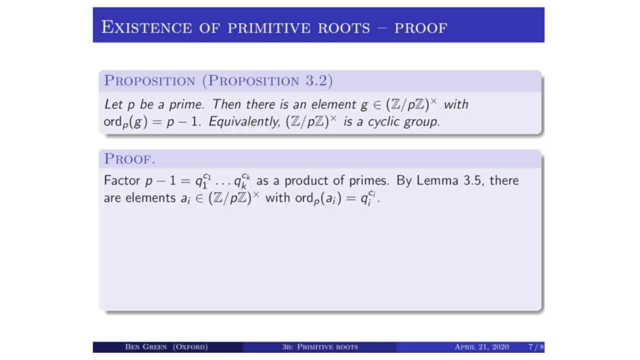 By the lemma on the last slide there are elements ai in z mod p, z star, with the order of ai mod p being qi to the ci. So for any prime power there's an element in z mod p, z star with that order. 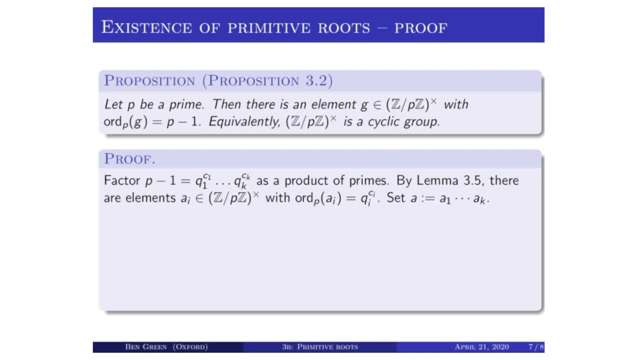 That's what we showed. Take a to be the product of those elements a1 times up to ak. Then the final lemma proven in section 3a was this one: lemma three, point three, It states that if I've got two elements, a1 and a2, of orders little n1 and little n2, modulo q. 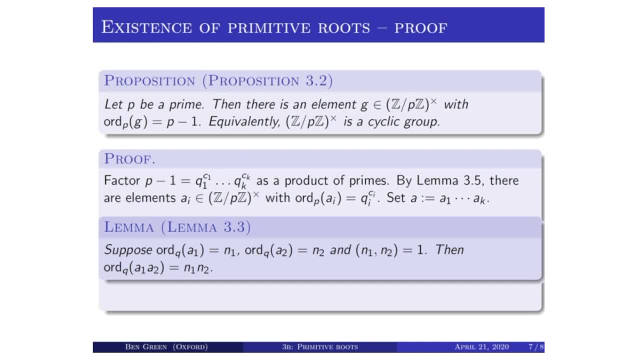 and if those orders are co-prime, then there is an element, specifically the product a1 times a2, whose order is the product of the little n i's And, if I apply this lemma here, with the product of all of the ai's. 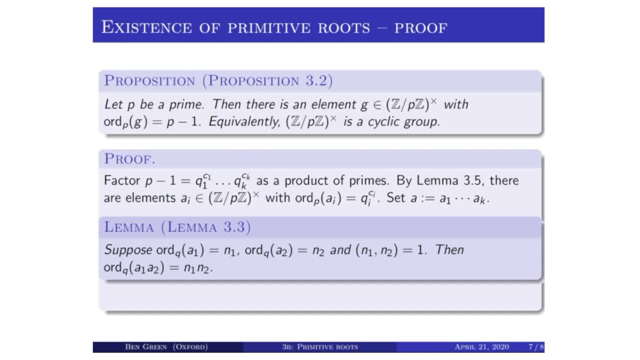 so if I apply the lemma repeatedly, what I get is that the order of a will be the product of the orders of the ai's. So the order of a- a being a1 times up to ak- is the product of the orders of the ai's. 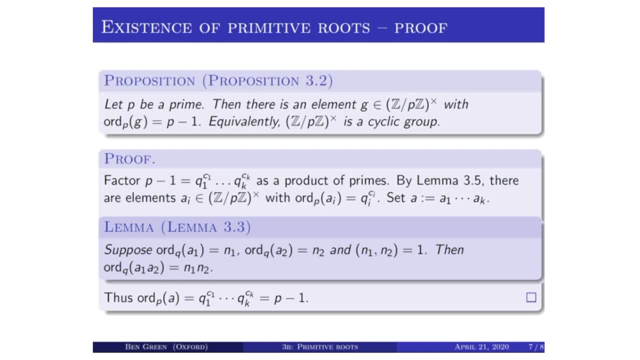 That is to say the product of the qi to the ci's, which by design, is exactly p minus 1.. So I have exhibited an element a whose order is p minus, That is to say a primitive route or a generator for z mod, p, z star as a cyclic group. 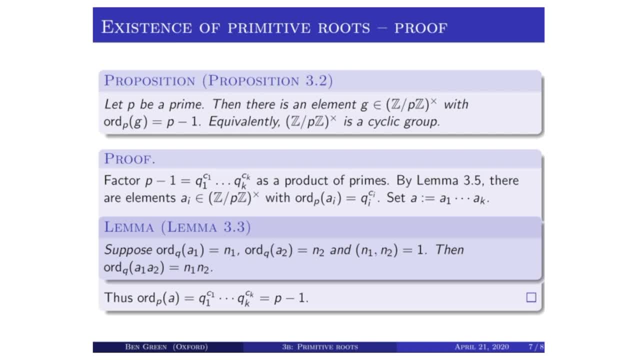 That concludes the proof of the existence of primitive routes, which was the main business of this section, And that tells us what the structure of z, mod, p, z star is as a group. It's a cyclic group of order p minus 1.. Now it's often useful to know: 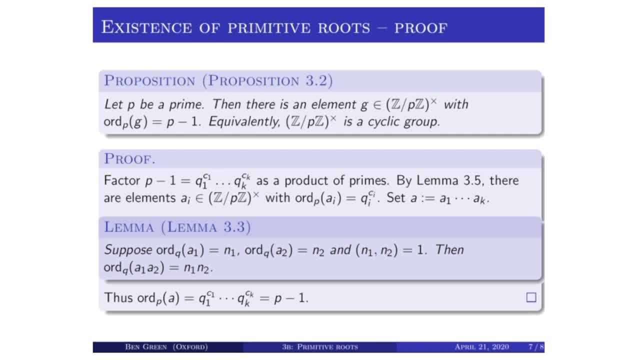 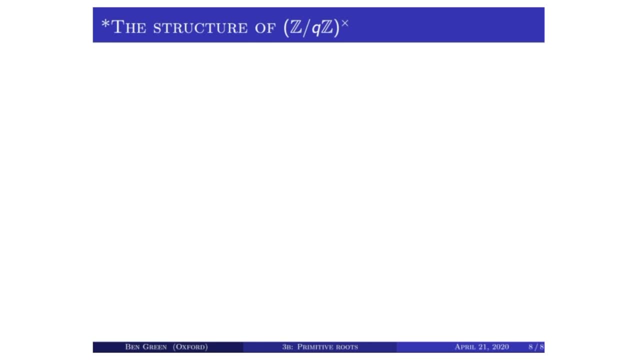 You might be a bit confused, Did you know? I'm not sure. I'm not sure. find yourself wanting to know what is the structure of Z mod, QZ, star for an arbitrary Q, And this is something that's not an examinable topic, but you'll find. 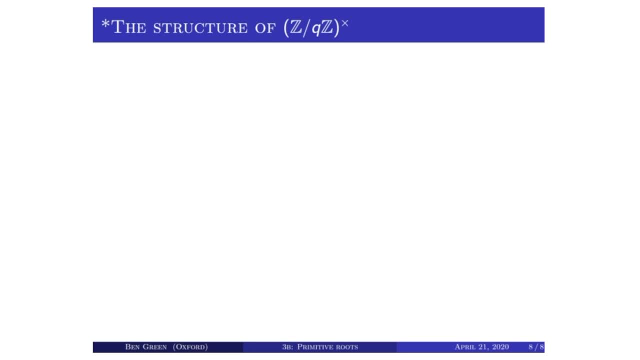 fairly full set of notes on it in the printed notes for the course. I'm not going to go over all of the proofs now, but let me just tell you what the crucial statements are. So this is about the structure of Z mod, QZ, star, where Q is not a prime. 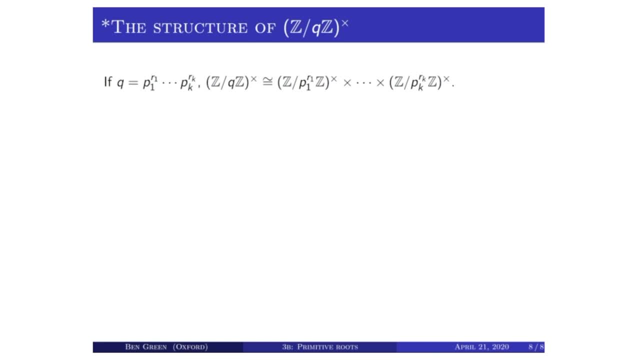 Well, the first thing to observe is that to understand the structure of that group, it suffices to understand what happens in the case when Q is a prime power, Because if I factor Q as a product of prime powers, then Z mod QZ star factors as the product. 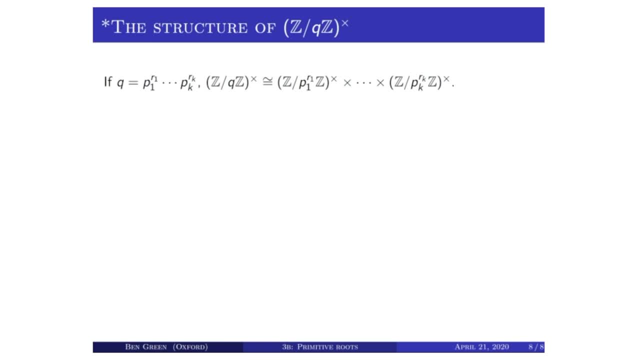 is isomorphic to the product of the Z mod, Pi to the Ri, Z stars, if Pi to the Ri are those prime power factors, And this follows from the multiplicative Chinese remainder theory. So it suffices to understand the prime power case. Now here's one key result about that. 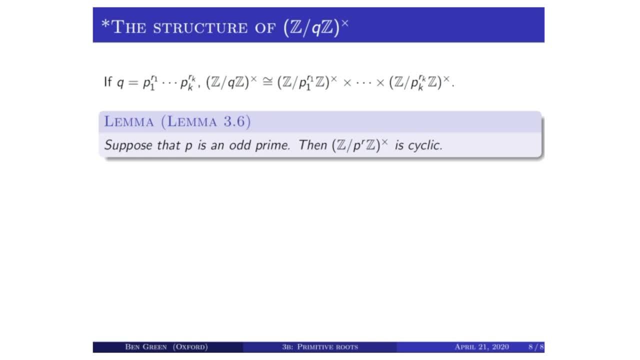 It turns out that actually primitive roots exist modulo odd prime powers. So this is a theorem, that is an elaboration of the existence of primitive roots modulo P, and the full proof you'll find in the notes. So if P is an odd prime and if R is an exponent, 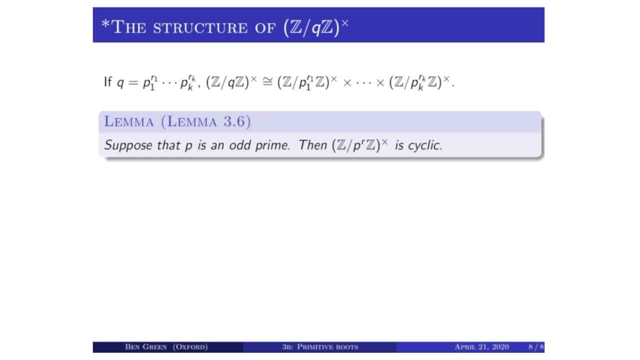 greater than or equal to one, then Z mod P to the R Z star is a cyclic group. And then there's a little wrinkle, which is that when P is not an odd prime, in other words when P is two, that's no longer the case. 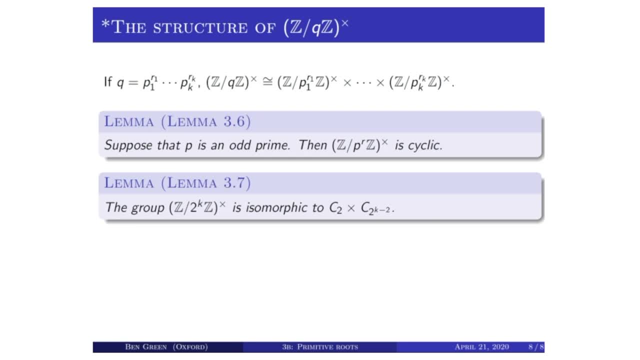 So Z mod two to the K Z star is not quite cyclic. It's isomorphic to the product of a cyclic group of order two and a cyclic group of order two to the K minus two. And again, you'll find a proof of this fact in the printed notes. 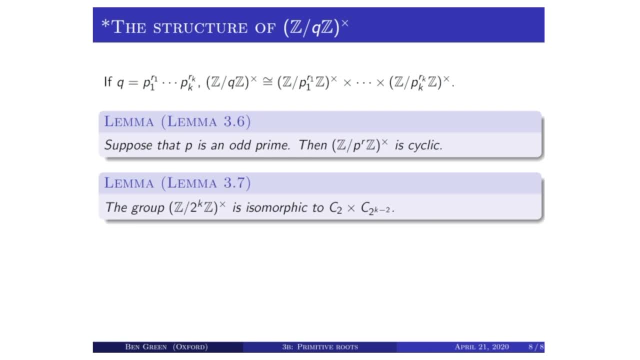 That cyclic group of order two to the K minus two, as it turns out, is generated by five. So five, while it's not quite a primitive root, modulo two to the K is as close to five as the root of root Q of the two. so it's not quite a primitive root. modulo two to the K is as close as that.